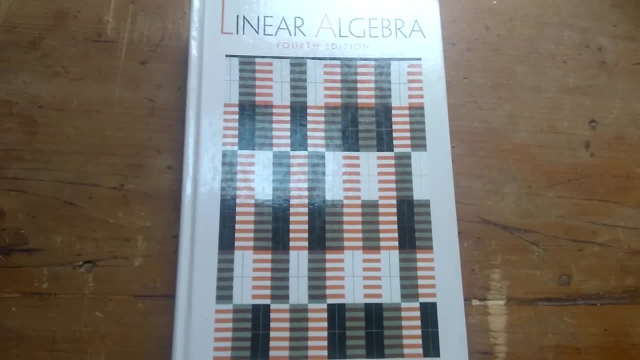 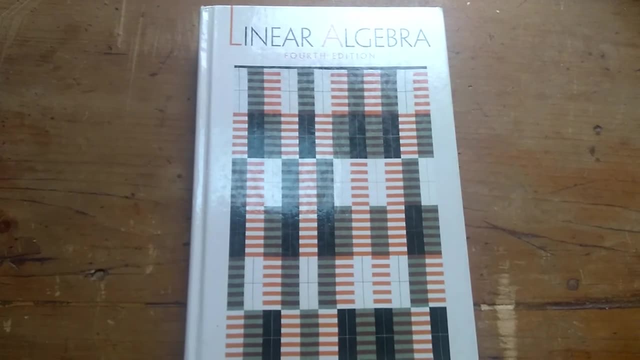 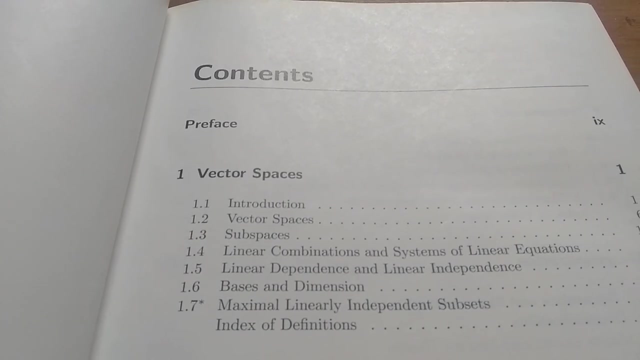 So I used this book for an upper-level linear algebra course many, many years ago, which I found incredibly difficult. Let's take a look inside this book. So what is good about this book? Well, I think the contents. That is the number one thing that is positive about this book is the contents. 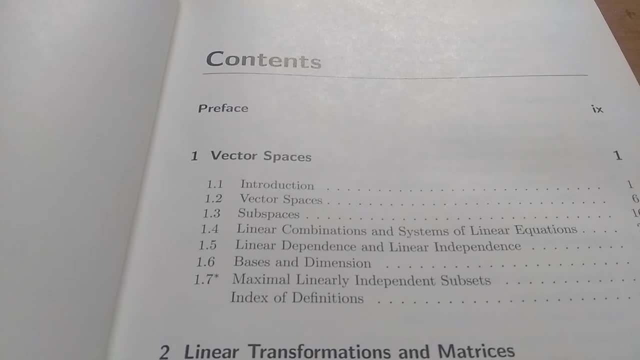 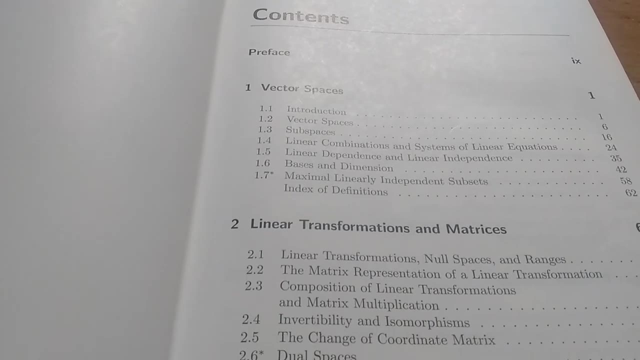 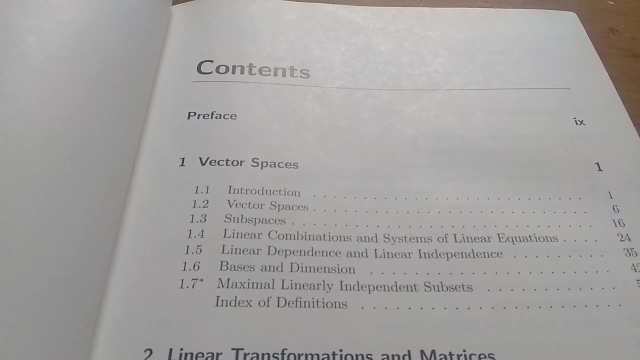 It contains so much information. In fact I would venture to say that this is the most comprehensive linear algebra book that I own, and I own maybe like four or five. So it starts off with vector spaces and the treatment is very axiomatic, Like it's very, very rigorous and it's very, very correct. 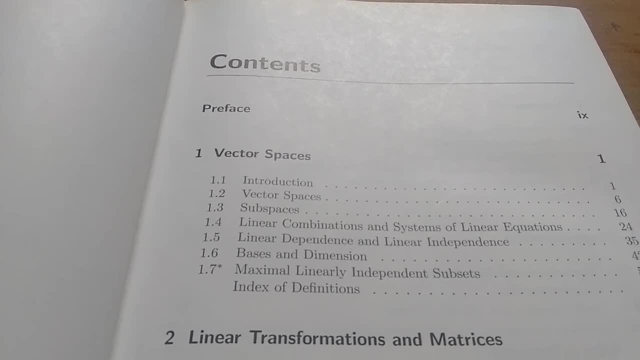 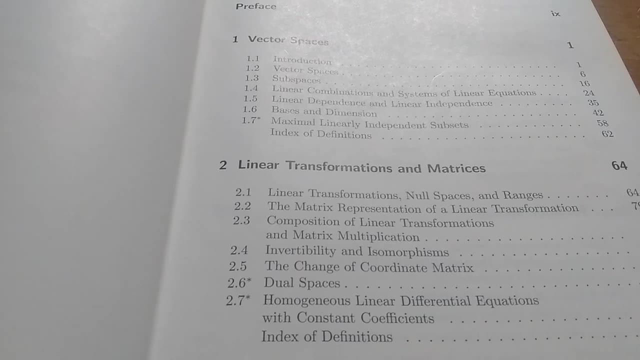 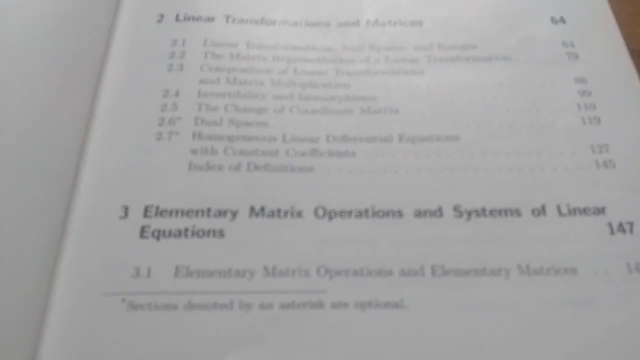 So it's a solid introduction, I guess you could say, into abstract linear algebra. Then he goes on to talk about linear transformations and matrices and again the treatment here is extremely, extremely rigorous. The third chapter is on elementary matrix operations and systems of linear equations. 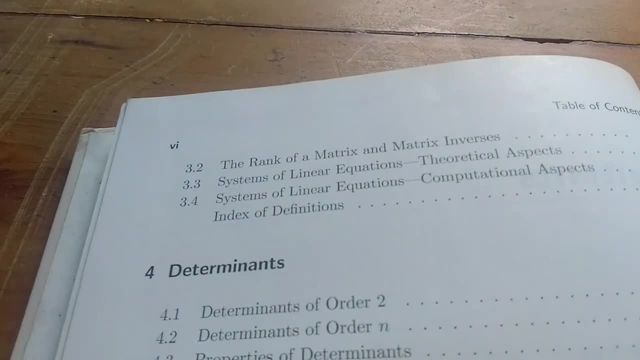 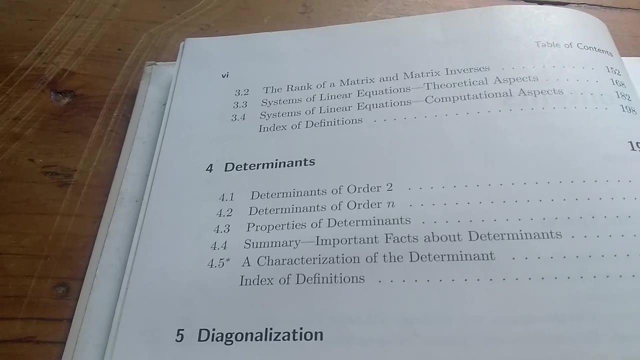 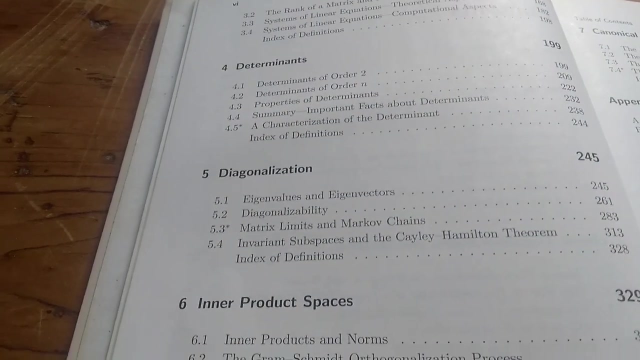 Turn the page. So he talks more about the rank of a matrix and matrix inverses and more on systems. Section four, or chapter four, is on determinants. Okay, Then five. he goes into diagonalization. So the book, if I recall, does contain all of the key theorems surrounding diagonalization. So if you're 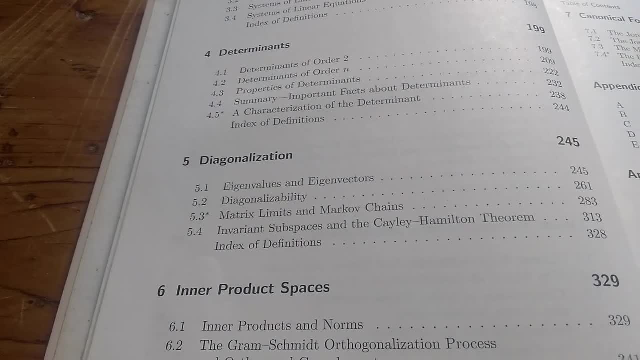 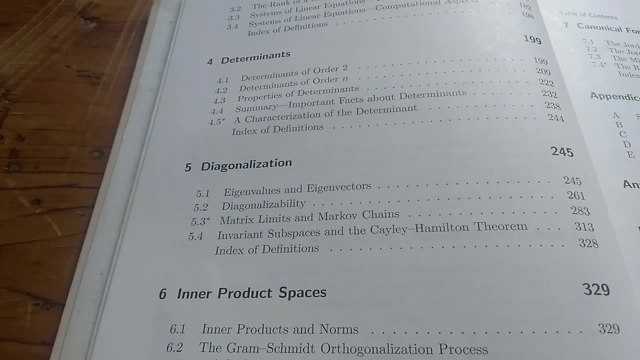 doing linear algebra in another course and you need to reference stuff. this is like the ultimate book because it has everything in it. It has all the theorems surrounding the minimal polynomial and all of that stuff. Then it goes on to inner product spaces. 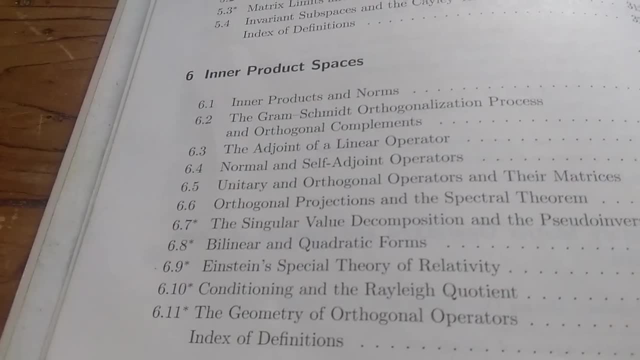 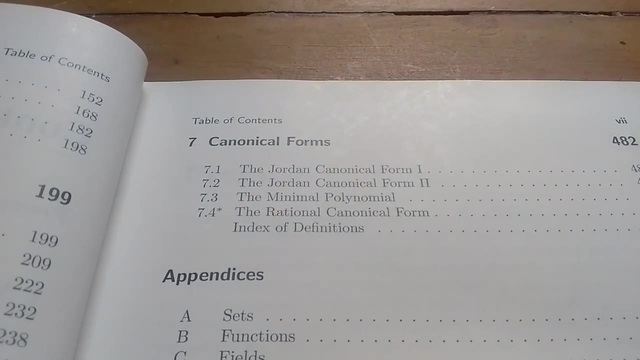 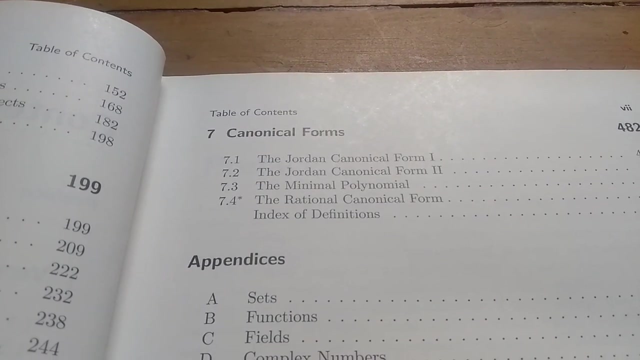 The chapters with the or sections of the little stars are considered optional. Then it goes on to the Jordan form. It's a pretty good treatment of the Jordan form. I have another book that I used to teach myself the Jordan form. I did not use this one to learn the Jordan form, but the treatment here is still pretty solid And 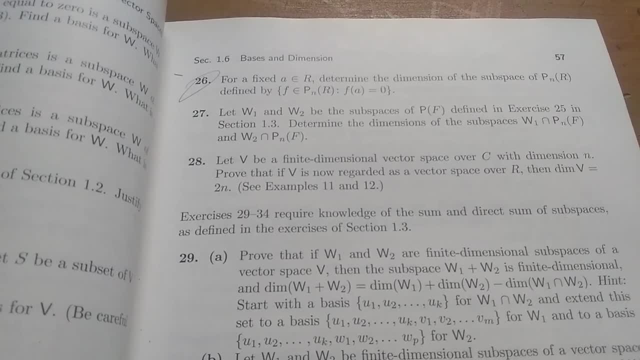 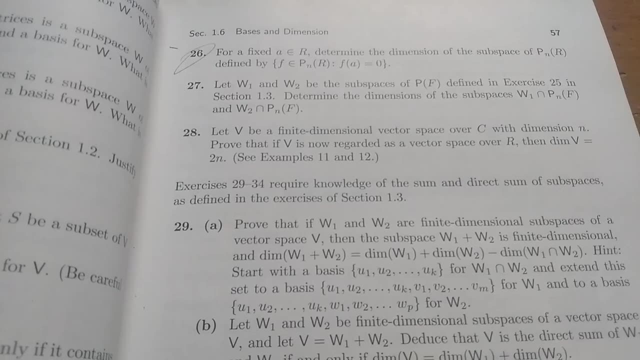 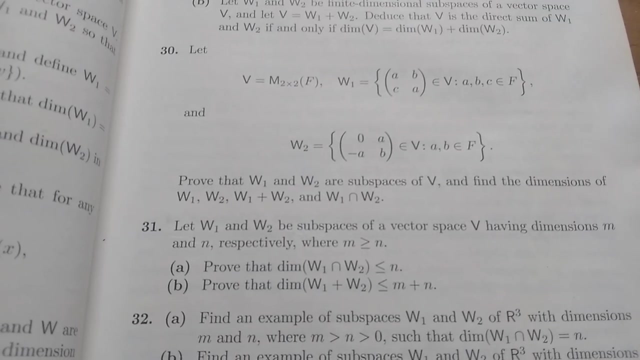 that's all of the contents. Another really positive thing about this book are the exercises at the end of each section. So Friedberg includes tons of exercises in each section. There are so many and a lot of them are not exactly very easy. So 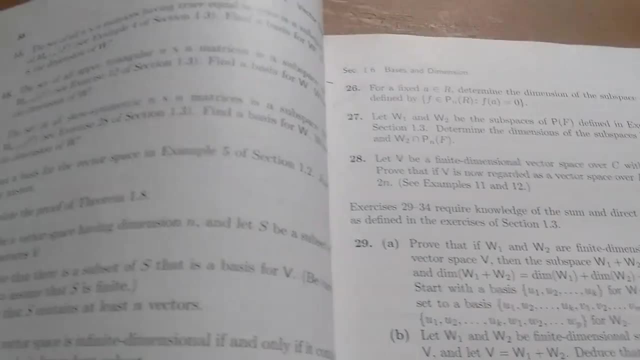 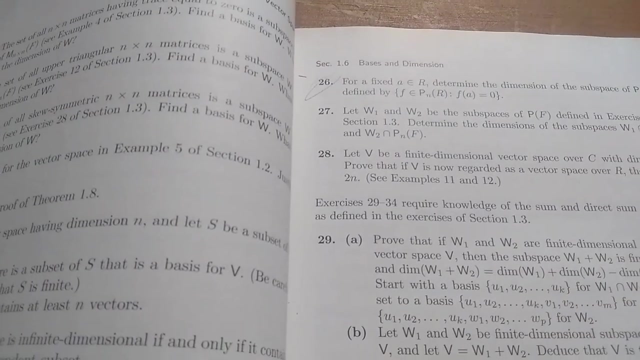 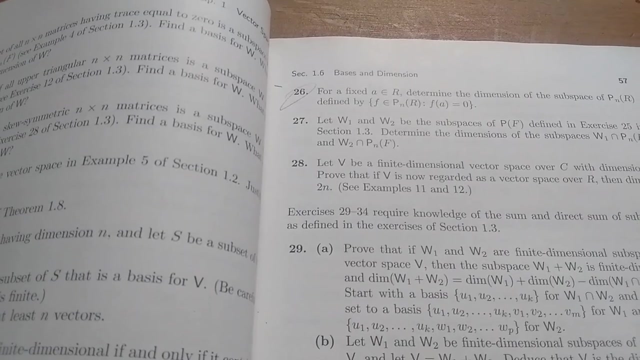 there's just tons of problems in each section. So if you're looking for linear algebra problems and proofs to do, this book has them. It's extremely comprehensive and, again, it has tons of exercises. So those are the two main positives for this book. Again, the comprehensiveness. 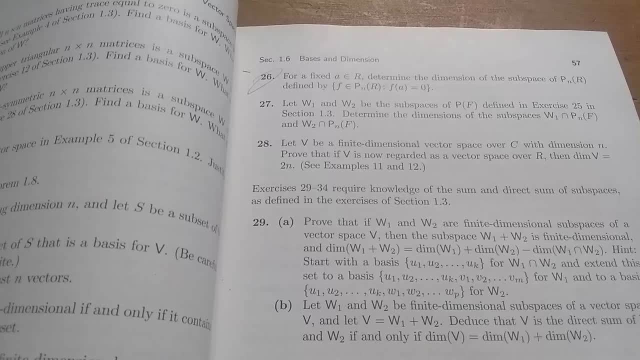 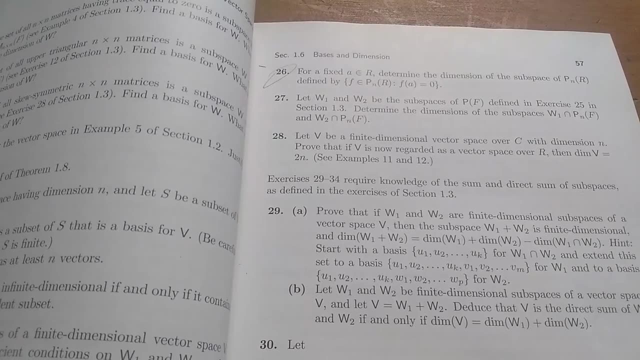 really allows you to like add it to your mathematical library and kind of have it as a reference, And that's what I've always used it for over the years. There's one more thing I want to talk about. The last thing worth mentioning about this book is the readability of the book. 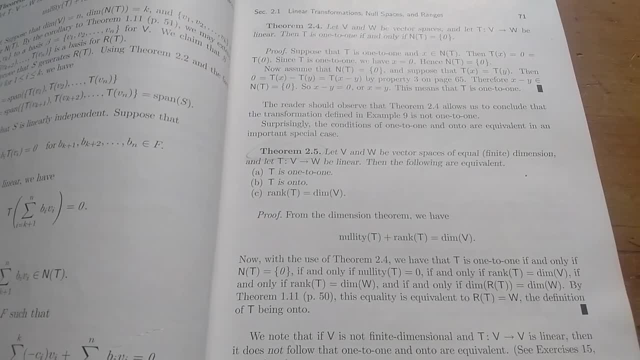 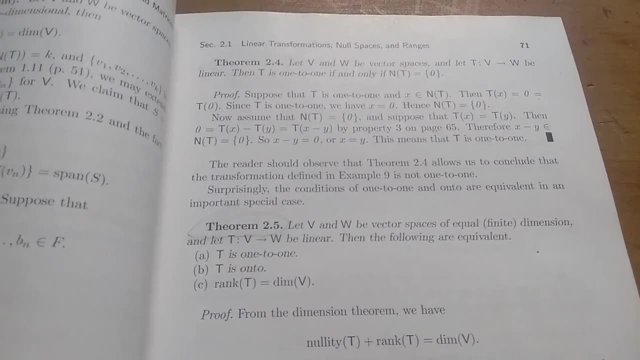 It's an okay book to read. I think it's a hard book to learn from. If you're reading this book, like any math book, you need to have a pencil and paper next to you as you read through it and as you try. 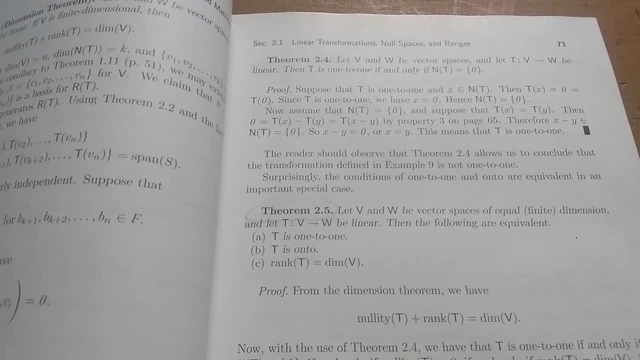 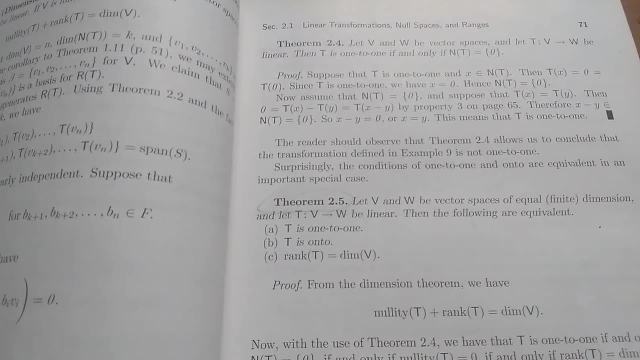 to learn the material, But this one in particular is a little bit harder to read than other math books. I have abstract algebra books that are easier to read than this linear algebra book, So I think the author writes some of the proofs in a way that. 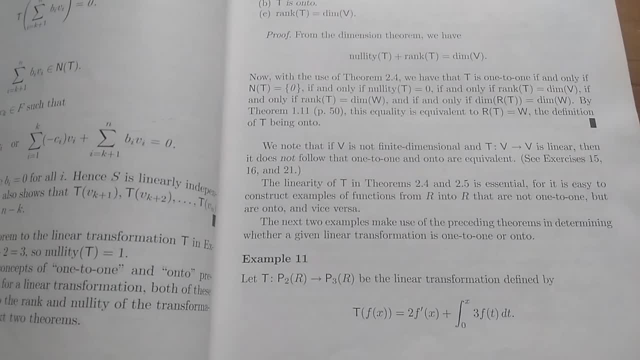 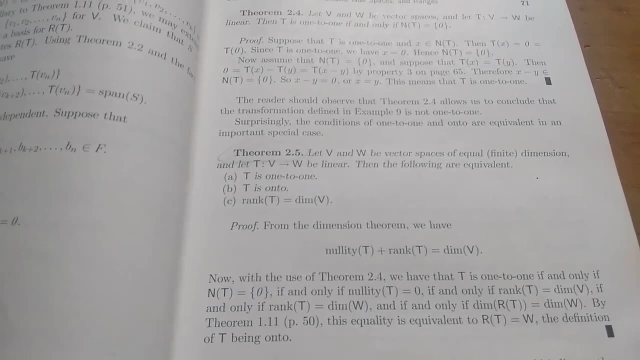 are just too complicated. I don't know if that's the right word. Maybe what I'm trying to say is: I feel like if you write your own proofs to the theorems as you go through the book, you will have a more enjoyable experience. So like, for example here, Theorem 2.5.. 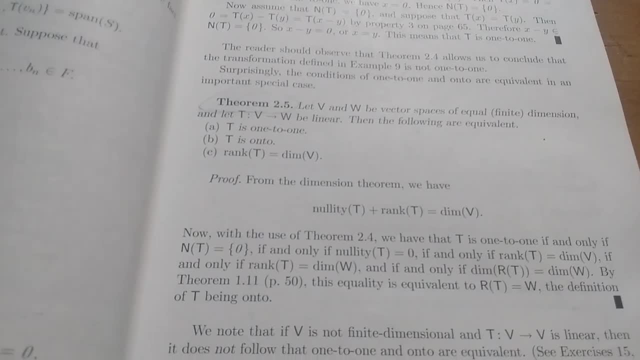 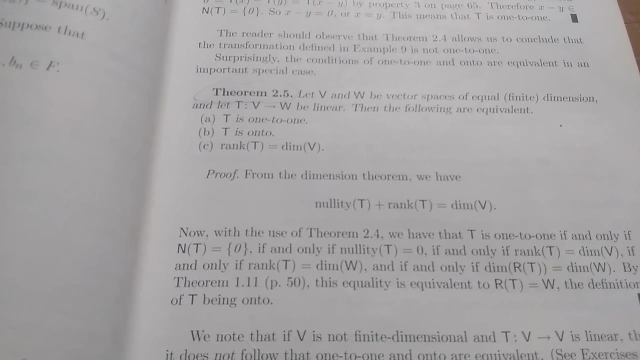 Try to prove this on your own before looking at the proof, and then, like you know, you glance at the author's proof and then you try to fill in the details yourself. It's always better if you do stuff on your own rather than just read the proof directly from the book. 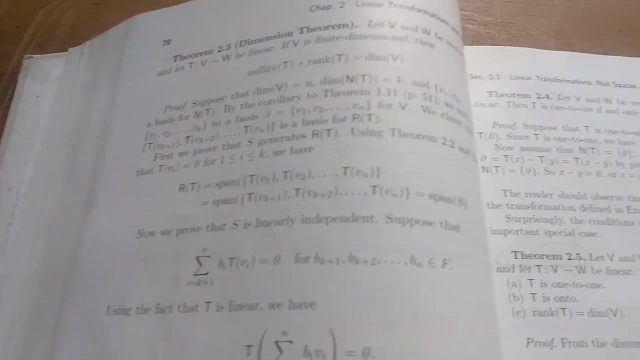 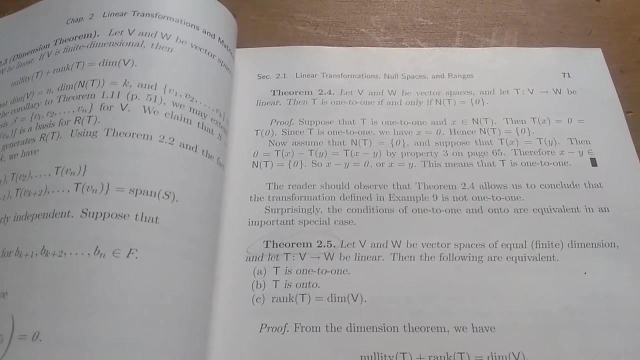 So overall it's a good book: Tons of exercises, extremely comprehensive, an awesome reference. But again, I think if you're gonna learn from this book, you really need to take a lot of initiative and try to write the proofs on your own. 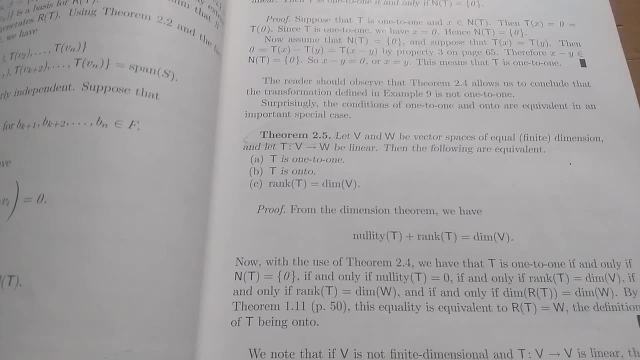 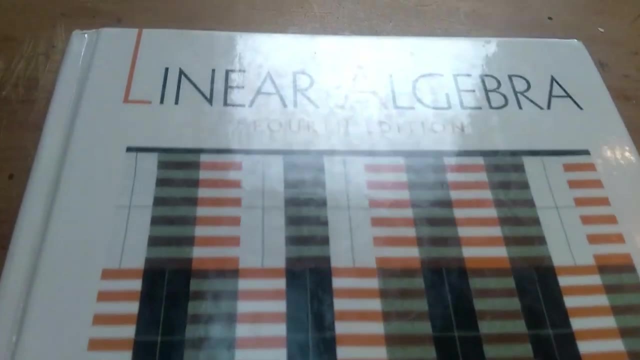 instead of reading them directly from the book. So I hope this video has been helpful to anyone out there looking for a linear algebra book. So again, the book is linear algebra and this is the fourth edition. I don't know if this is the latest edition. 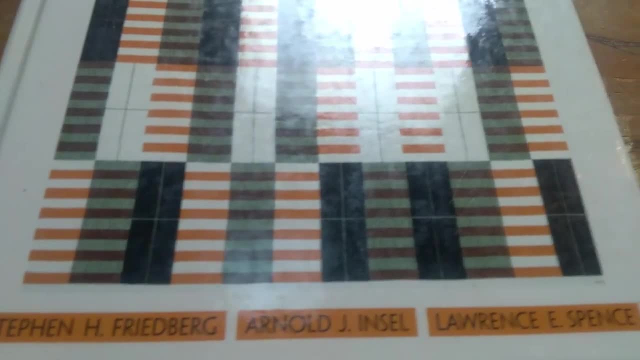 It probably isn't, And the author is Friedberg, Insell and Spence. Those are the authors, That's it.